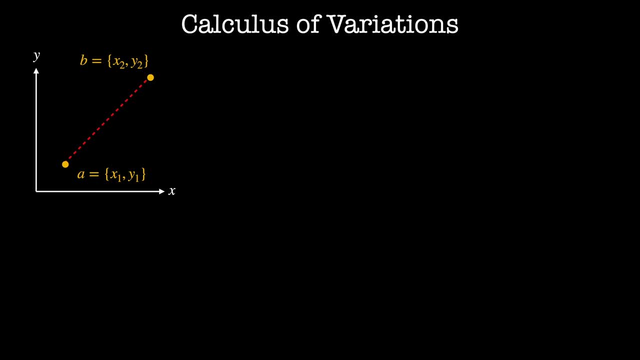 between a pair of points is a straight line, but can we prove it? This is what the calculus of variations teaches us to do. We'd like to minimize the length of a path that goes from point a at x1- y1 to point b at x2- y2.. The catch is, though, that I can have any path I'd like We want to. 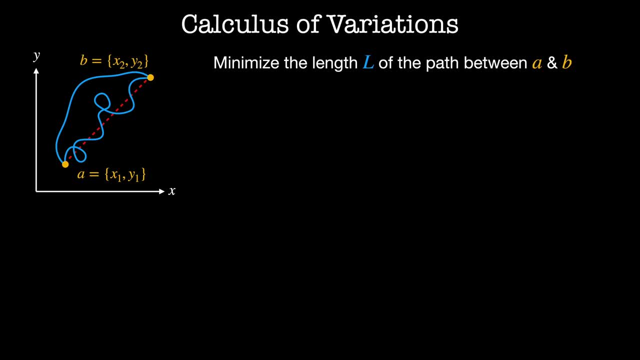 figure out which path of all possible paths is going to be the shortest. Let's write a generic path as y as a function of x and the total length of the path y is equal to the integral, from x1 to x2, of the square root of 1 minus y, prime squared d- x. We want to figure out how to minimize this. 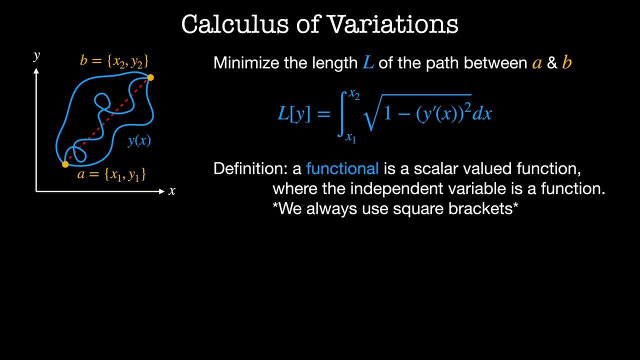 length l. l is what we call a functional. A functional is a scalar valued function where the independent variable is itself a fact function, and the convention we use is that the argument of a functional is always in square brackets. Our path: length l is a functional of y. We're looking to find the extremal function. 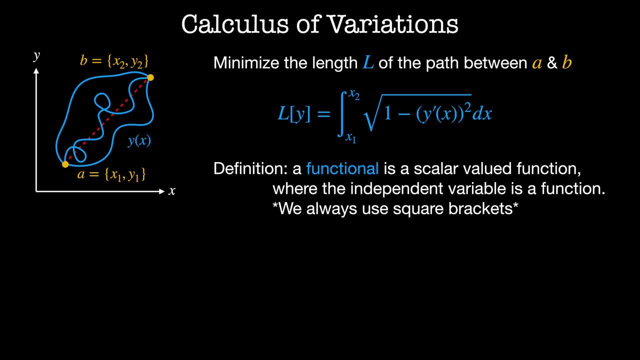 y of x. that minimizes the functional l. The calculus of variations enables us to find extremal functions as opposed to single variable calculus, where we find maximal or minimal numbers. In general, we'll always be looking to minimize some sort of functional. For example, i is a. 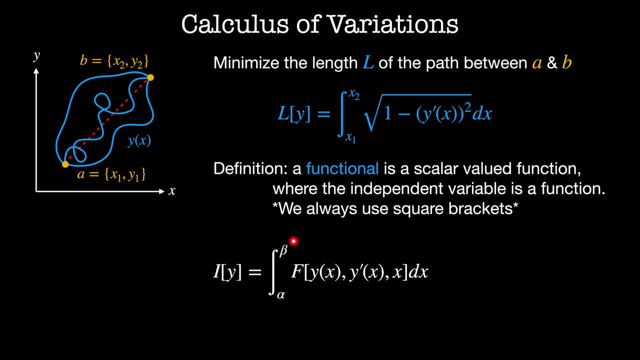 functional of y, which is the integral from alpha to beta of f, is a functional of y, of x and y prime of x, but it's also a function of the variable x. In physics this functional is often some sort of energy. For instance, in the soap film example, the energy is a surface tension. 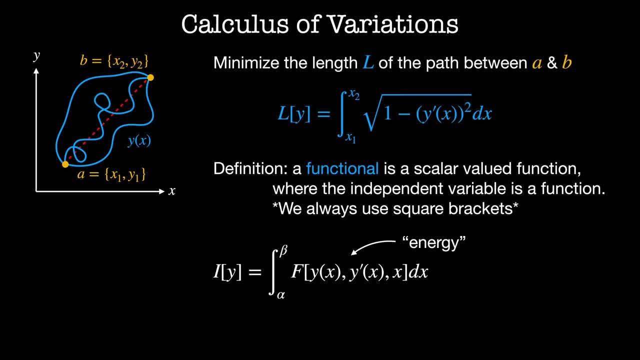 which is given by the surface area times an energy per unit area. Our goal is to figure out how to minimize some sort of functional, For example, in the soap film example, the energy is a surface area times an energy per unit area. Our goal is to 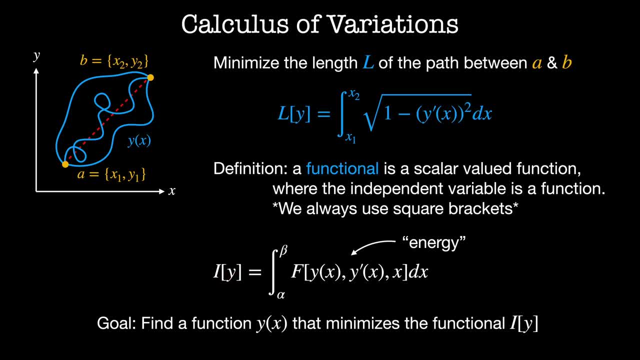 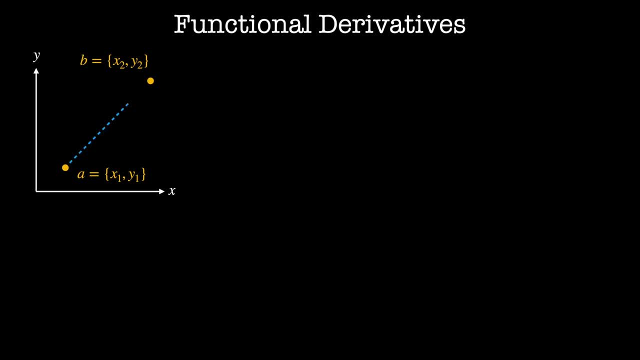 find a function y that minimizes the functional i. How might we make this mathematically rigorous? Let's start by assuming that a solution exists, For example the shortest path between two points. We'll call it y of x. To this solution, I'm going to add a tiny perturbation to it: Our 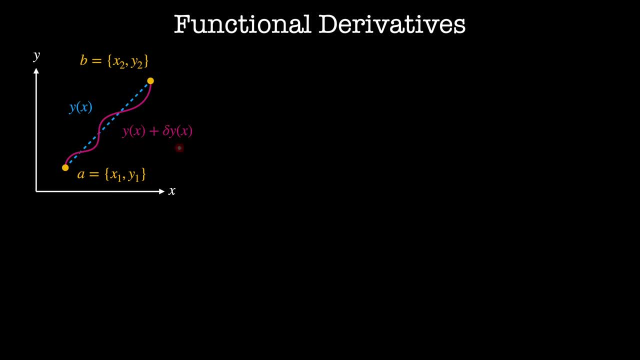 new curve is called y of x plus delta y of x, where delta y is a function and it has boundary conditions such that delta y at point a is zero and delta y at point b is zero. Now let's look at the difference between the energies of these two paths. Delta i is equal to 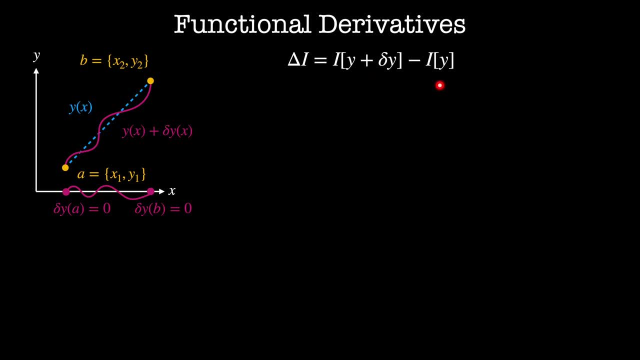 i of y plus delta y minus i of y. The energy of i of y plus delta y is greater than the minimal energy i of y. If y minimizes i of y, then in the limit that delta y goes to zero, delta i is equal to zero. This looks a bit like the formal definition of a derivative. 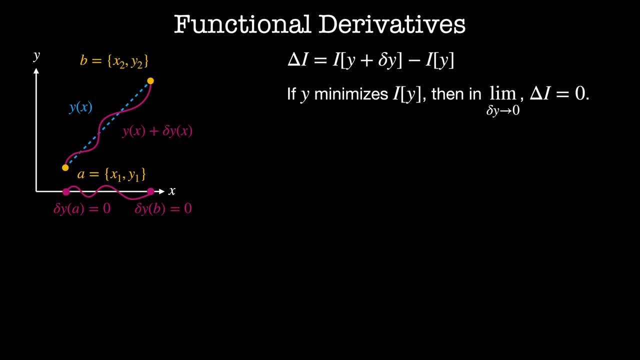 Let's expand out delta i and see how this analogy plays out. First, I need to expand the term f of y plus delta y y prime, plus delta y prime and x in terms of delta y and delta y prime. To do this, let's look at how to expand a function of two variables. 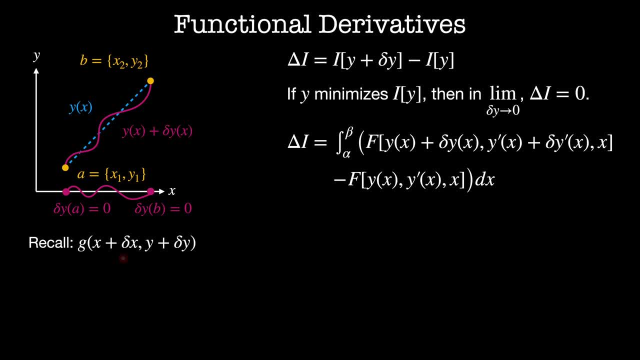 For example g of x and y, for small delta x and small delta y. This is just a formal Taylor expansion for a function of two variables: g of x plus delta x and y plus delta y is equal to g of x and y. 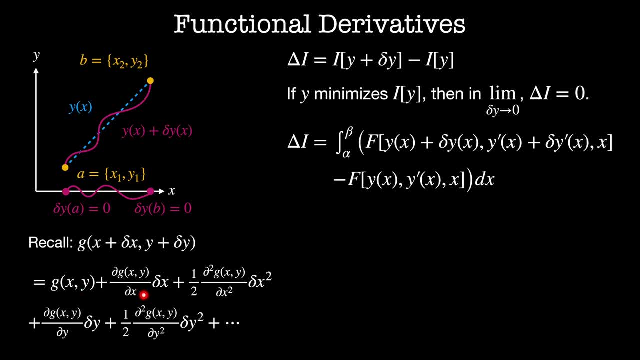 Now we have a linear term, dg by dx times delta x, plus a quadratic term, one half d squared, g by dx squared times delta x squared, And that's our expansion in terms of delta x, And we get an equivalent expansion in terms of delta y as well. We could include higher order terms, but it turns. 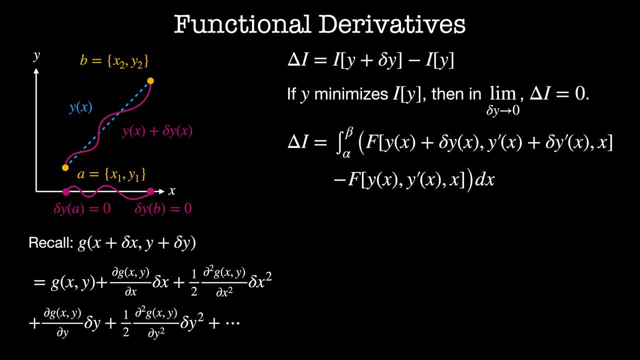 out that linear order is sufficient for our purposes here. Now we'll write out the expansion for f, for small delta y and for small delta y. For the first term we obtain the equivalent of delta x plus delta y plus f, of y, of x, y, prime of x and x. 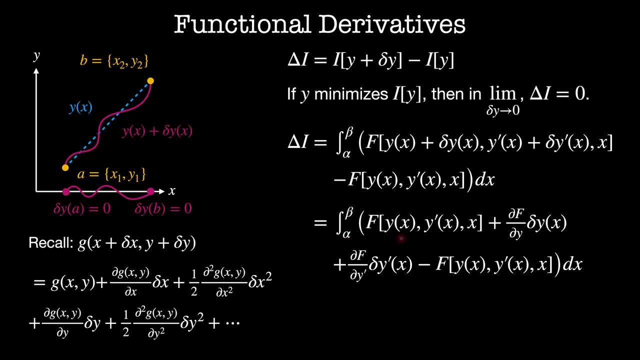 plus the linear term in delta y of x which has coefficient df by dy plus df by dy, prime times. delta y, prime of x, minus f of y of x, y prime of x and x dx. First and last terms: cancel out. 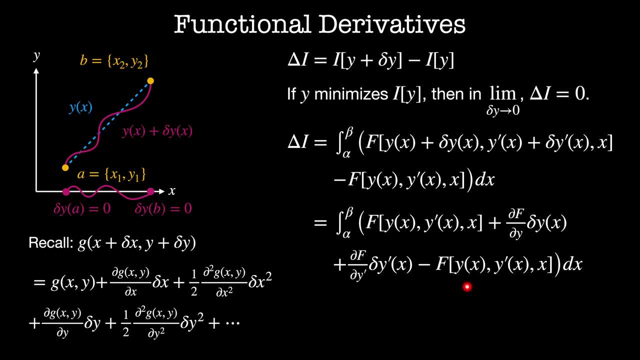 and we're left with the integral f of y of x, y prime of x and x dx. Now you can mark this and see that this is the same formula for f of y of x, y prime of x and f of x of x. 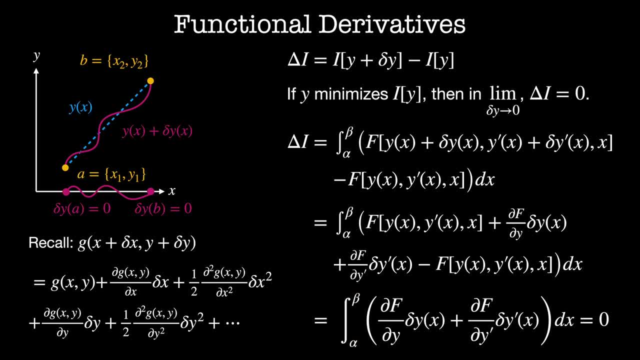 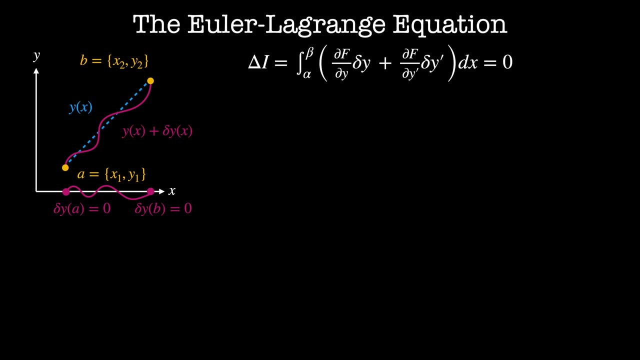 integral from alpha to beta of df by dy times delta y of x plus df, by dy prime times delta y, prime of x dx, which equals zero if y of x minimizes i. Next we'll figure out what to do with this term here. The first thing we'll do is take the second term and integrate it by parts. 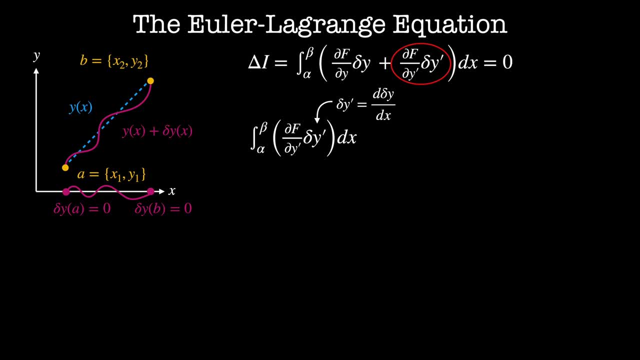 We can write delta y prime as the derivative of delta y with respect to x. Quick aside, the derivative I just took uses d's rather than partial derivatives, because delta y is only a function of x. The derivatives of f, though, use partial derivatives, because f is. 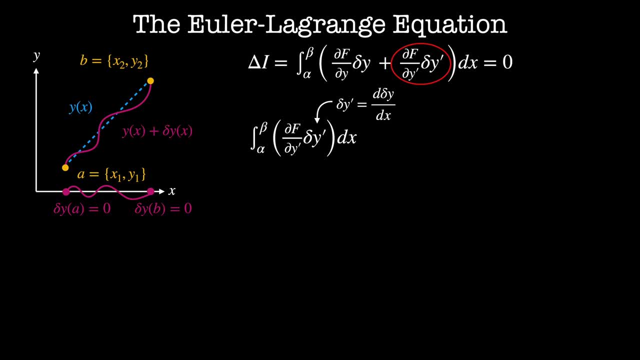 treated as if it were a function of three independent variables. So those would be y, y, prime and x. Now let me integrate this by parts. The integral of udv is equal to uv, evaluated at the boundary points, minus the integral of vdu. We're going to do that on this right here, The first term. 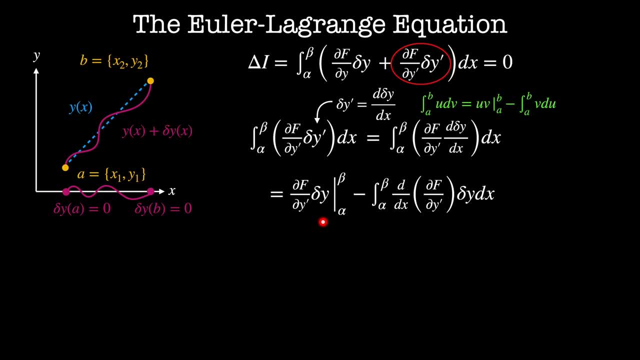 is df by dy times delta y evaluated at alpha and beta minus the integral from alpha to beta of d by dx, of df by dy prime times delta y prime times dx. The first term over here vanishes because delta y evaluated at either of the boundaries equals zero by definition. 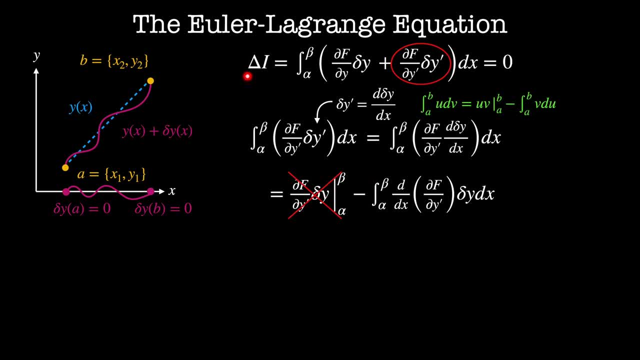 And we're left with this. Let's continue learning delta x from alpha to beta as we begin. And why is this going to take so long? The first thing to do is plug in a common interval on f, which we know is delta x. 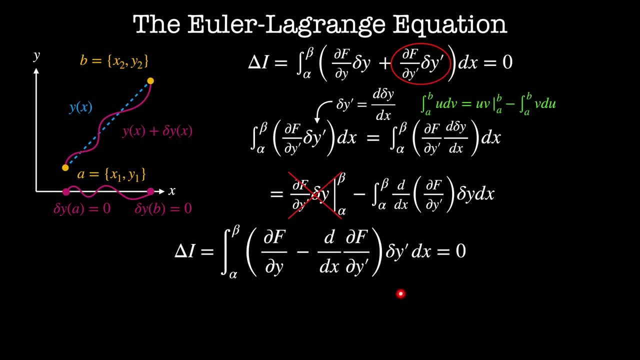 Then plus f, twice delta y times delta y d is theца, which is equal to the integral from alpha to beta, minus f, which is exactly the equal to the integral from across the grid. We just want our equations to work for now. Let's save the Espa ph of this integral here. Let me plug that into the definition for delta i. I get: delta i is equal to the integral from alpha to beta of the partial derivative of f with respect to y minus d by dx of the partial derivative of f with respect to y prime times delta y prime times dx. 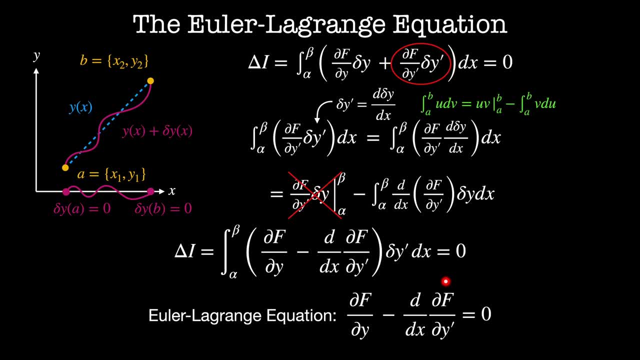 And this whole thing is equal to 0.. And this is called the Euler-LaGrange equation. d by dx of df by dy, prime is equal to zero. Finding the function y of x that minimizes the functional i comes down to solving this differential equation with the appropriate boundary conditions. 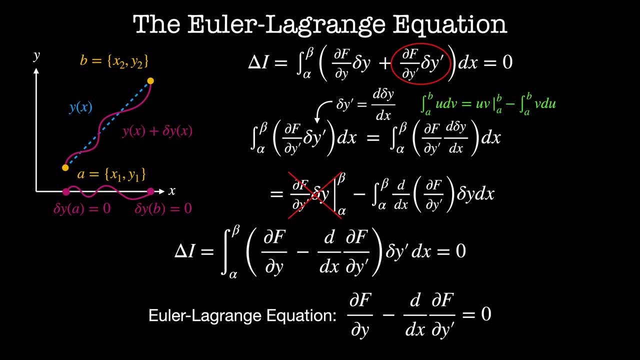 I'll leave it as an exercise for you to show that the shortest distance between two points in the plane is a straight line, using the definition for the path length as your functional f. One of the things that makes variational calculus so powerful is that we have a lot of flexibility. 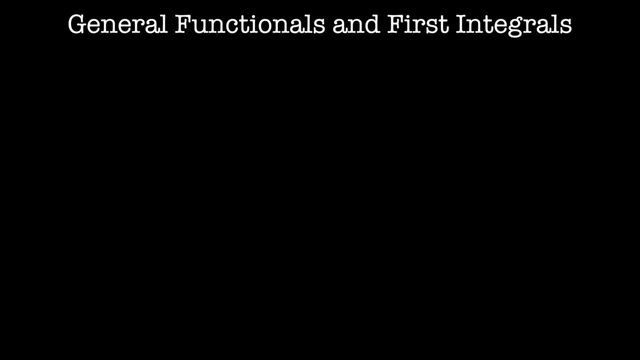 with our coordinates. In the previous example I wrote y as a function of x, but I could equally well have written x as a function of y or r as a function of theta, And in all cases, solving the Euler-Lagrange equations would have given us a straight line in each of our coordinates. 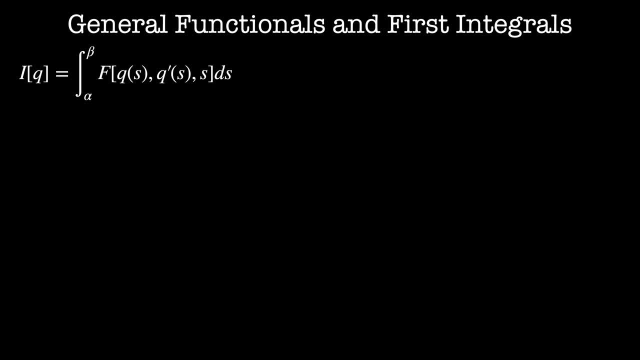 If we have general coordinate q as a function of our parameter s, then our functional looks like this: i is the integral from alpha to beta of the functional f, which is a function of q, of s, q, prime of s and s, ds. Then the Euler-Lagrange equation is the partial derivative. 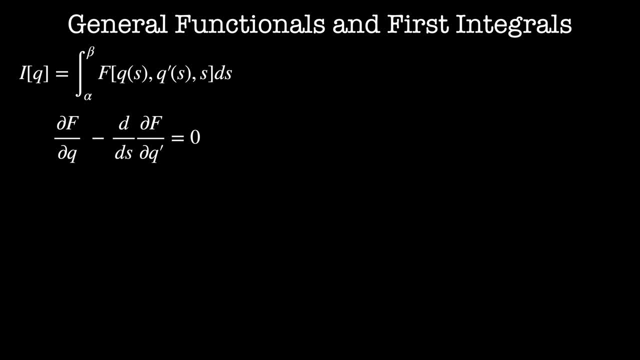 of f with respect to q, minus d by ds of the partial derivative of f with respect to q, prime, and this is equal to zero. Or I can rewrite this, which is slightly more common, as the partial derivative of f with respect to q is equal to d by ds of the partial derivative of f with respect. 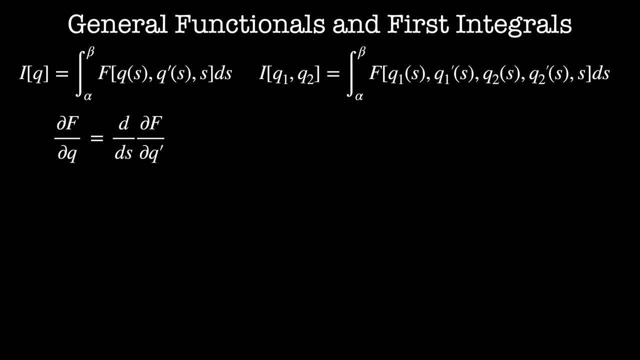 to q prime. We can also write a functional in terms of more than one generalized coordinate. Here our functional f depends on q1 of s, q1 prime of s, q2 of s, q2 prime of s and s. And if this is, 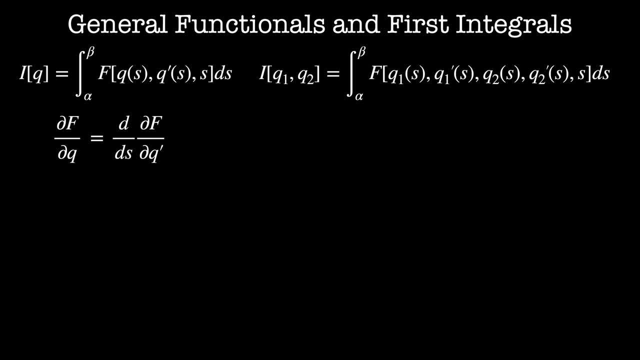 the functional that we're trying to extremize. we have two Euler-Lagrange equations we need to solve, And these are: the partial derivative of f with respect to q1 is equal to d by ds of the partial derivative of f with respect to q1, prime. 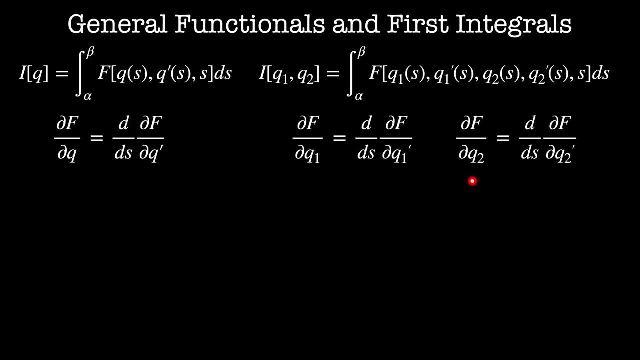 And the other one is: the partial derivative of f with respect to q2 is equal to d by ds of the partial derivative of f with respect to q2, prime. Solving both of these together gives us a pair of functions which extremizes the integral i. Next let's take a look at a couple of special 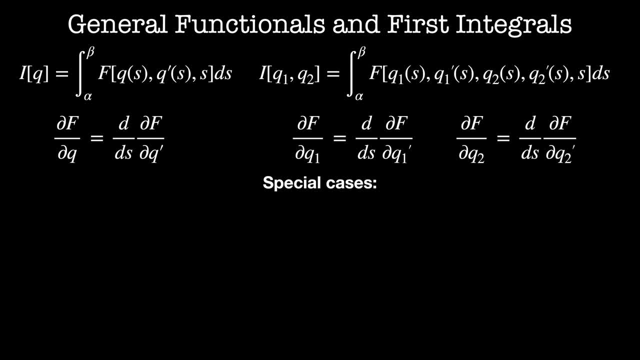 cases that make integrating the Euler-Lagrange equations easier. These special cases give us so-called first integrals for our equations. In these cases we can write the Euler-Lagrange equations as total derivatives of our parameter s. For the first case, if the function f does not, 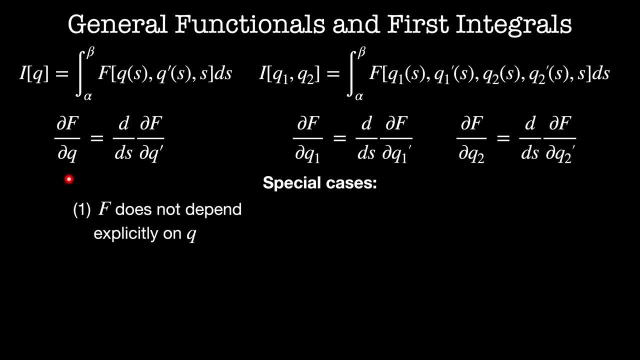 depend explicitly on q, then this term, here the partial derivative of f with respect to q- is equal to 0. Then d by ds of the partial derivative of f with respect to q prime is equal to 0. And we can integrate this so that the partial derivative of f with respect to q prime is now a. 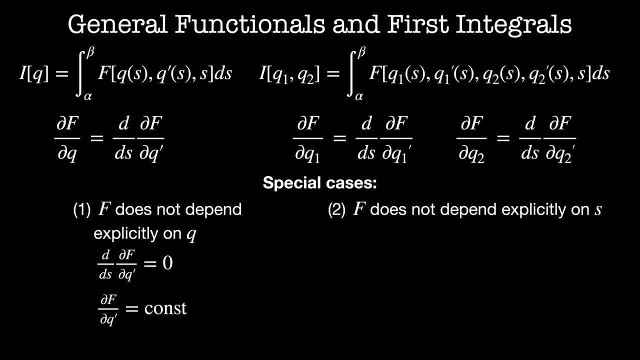 constant. The other case happens when f does not depend explicitly on the parameter s. In order to see how this helps us, let's write down: the total derivative of f with respect to s df by ds is equal to the partial derivative of f with respect to s, plus dq by ds times the partial derivative. 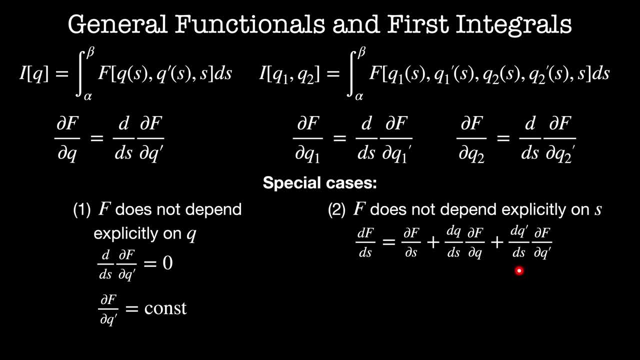 of f with respect to q plus dq prime. by ds times, the partial derivative of f with respect to q prime. Partial derivative of f with respect to s vanishes because f does not depend explicitly on s From the definition of the Euler-Lagrange equation. we can replace the partial derivative of f with: 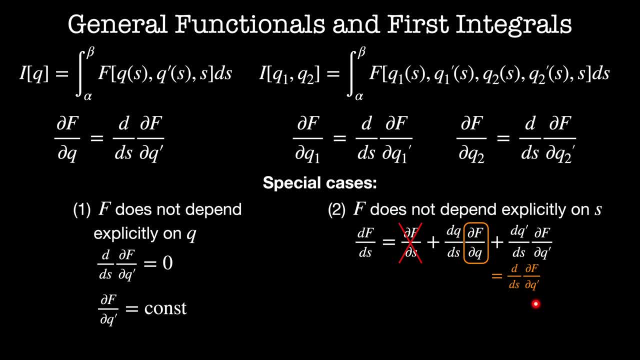 respect to q, with d by ds of the partial derivative of f with respect to q prime. Next thing I'm going to do is undo the chain rule on these two terms and I can write this as a total derivative of s, And so this is equal to d by ds of q prime times the partial derivative of f, with 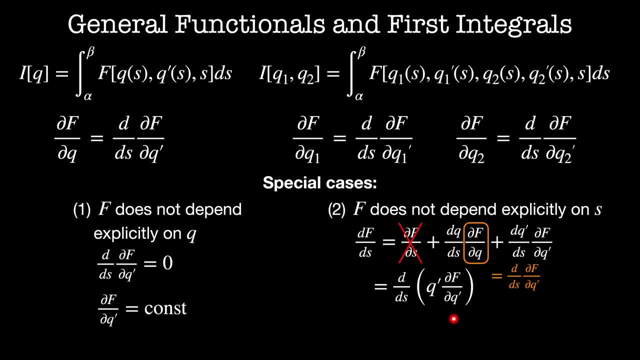 respect to q prime, And this whole thing here is equal to the total derivative of f with respect to s. Now I can collect terms and I get d by ds- of f minus q prime times the partial derivative of f with respect to q prime, and that whole thing is equal to zero. Or, when I integrate it, f minus q.